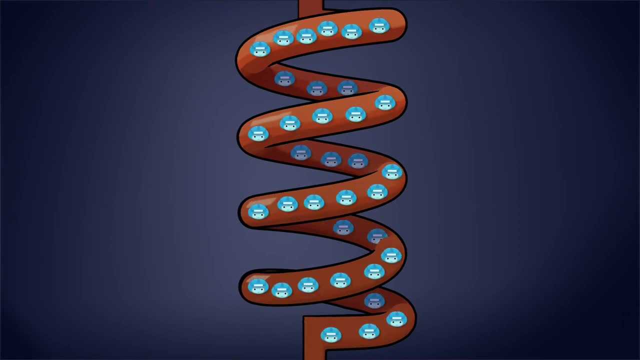 to their atoms. So these electrons are bouncing around all over the place in the copper. Since the electrons are moving randomly, there is no electrical current in the wire normally. But when a magnet is moving close to the copper wire, the tiny electrons in the copper wire get. 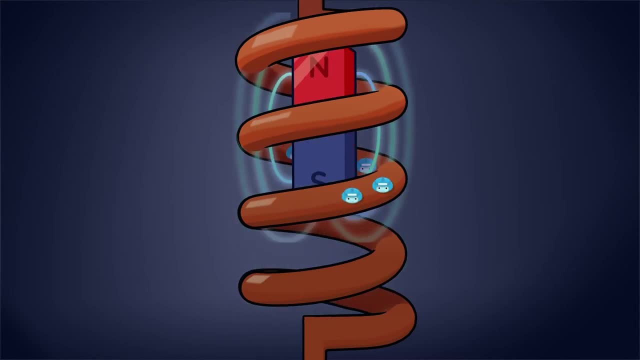 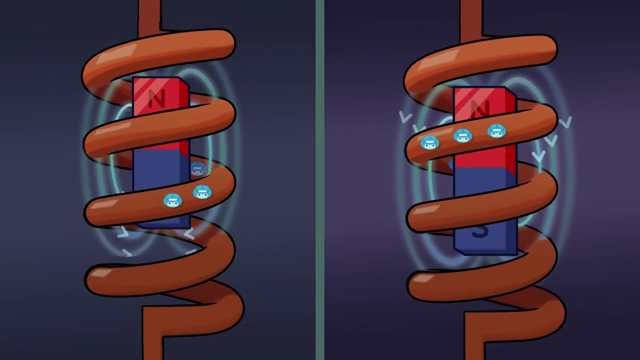 pushed by the magnetic field, These electrons move together and electrical current is generated. A steel magnet has no such effect. It's the changing flux of the magnetic field that gets the electrons to move together. It doesn't matter if the magnet moves or the copper moves Either way. 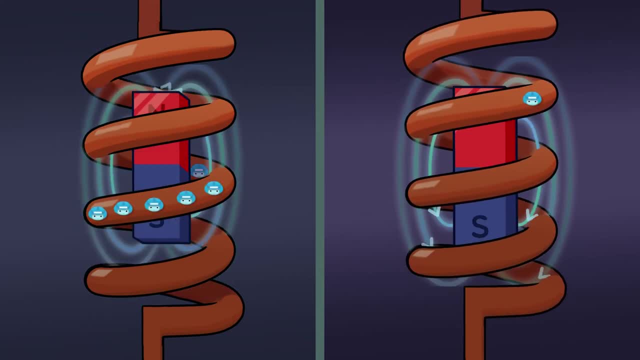 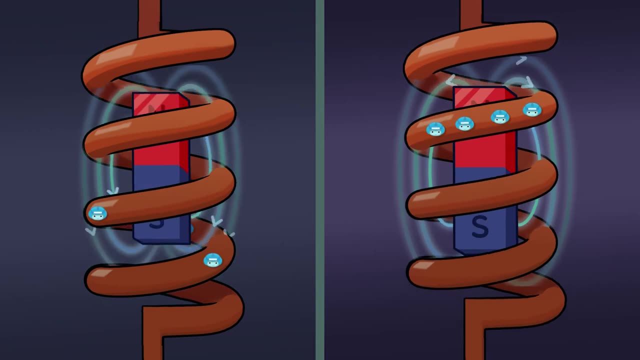 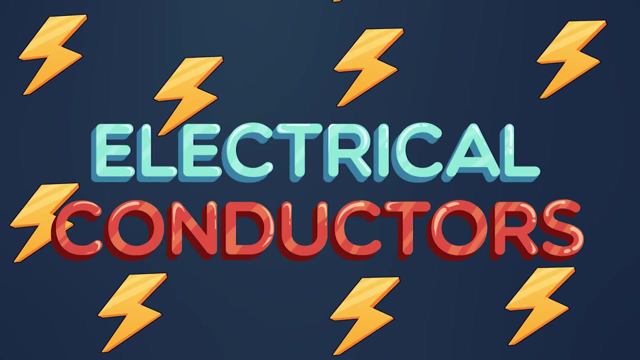 the electrons in the copper wire get pushed by the changing force of the magnetic field and electrical current is created. Only certain materials respond to magnets this way, Only metals, especially copper, silver and gold. These metals are called electrical conductors. 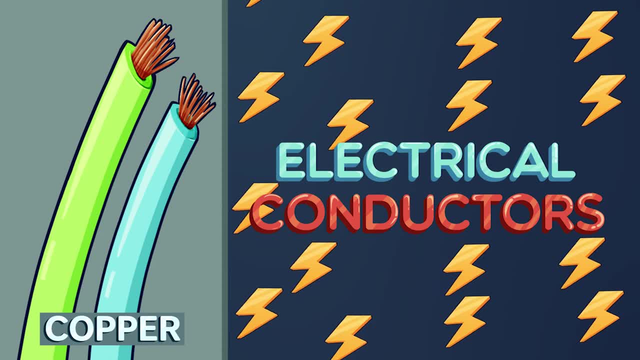 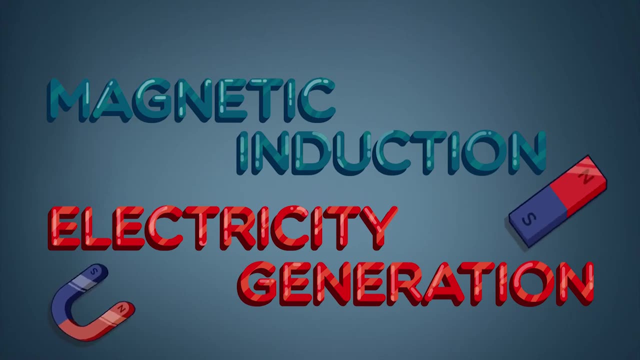 Copper is the cheapest, so it gets used the most. Since the magnetic fields don't change to copper, they only induce the electrons to move in the wire. This form of making electricity is called magnetic induction electricity generation. It's used in all sorts of ways like wind power. 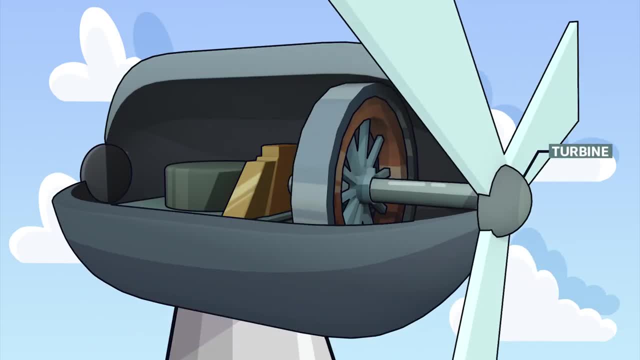 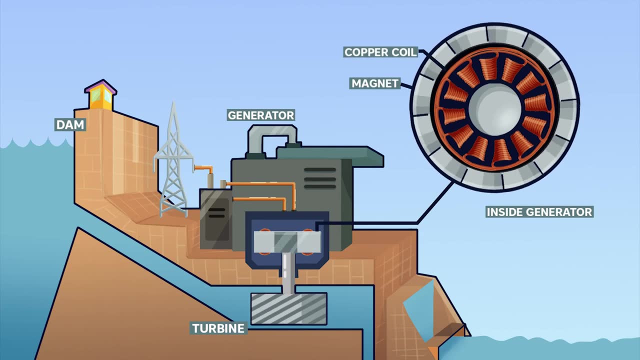 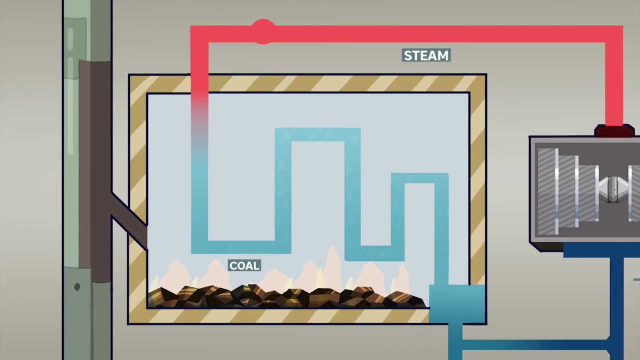 The wind moves the blades which rotate strong magnets near copper coils, generating electrical current In hydropower. flowing water moves a turbine which spins magnets near copper coils, making electricity. Coal-fired power plants burn large amounts of coal to boil water and make steam. 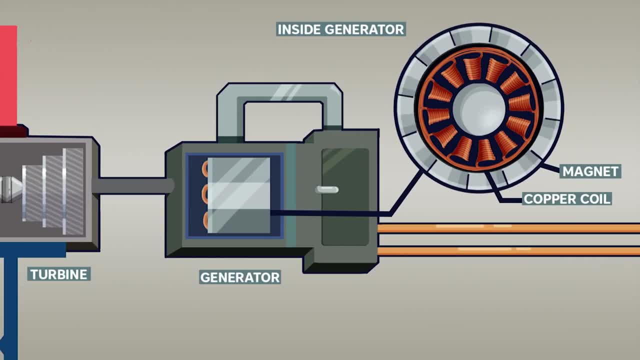 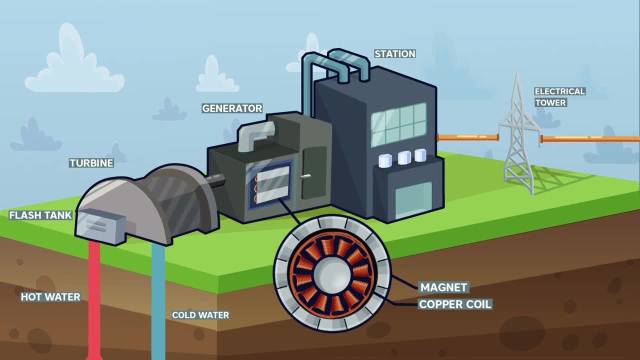 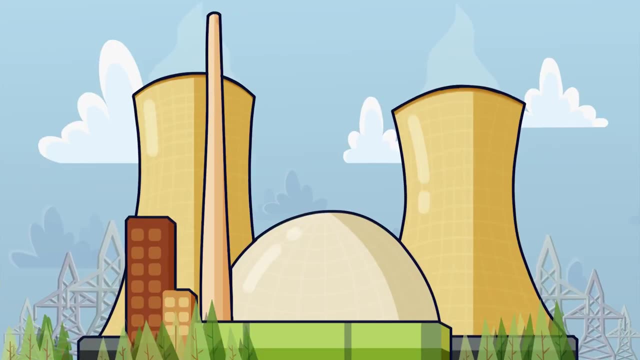 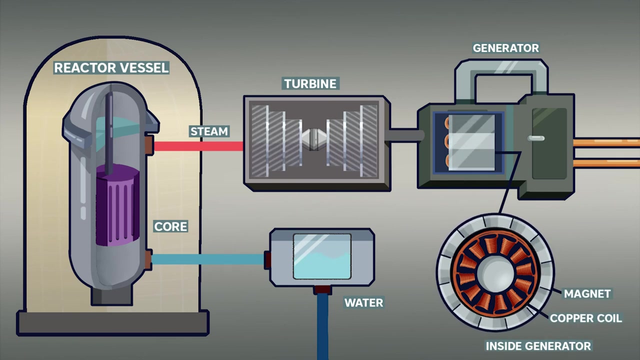 which turns a turbine to spin- you guessed it- magnets around copper coils. Geothermal power plants use the heat deep inside the earth to boil water, producing steam that turns turbines which spin magnets around copper coils. Even nuclear power plants work by using the heat of atomic fission to boil water and make steam to turn magnetic induction turbines. 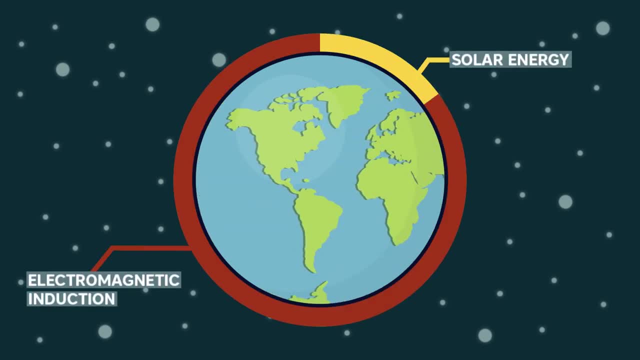 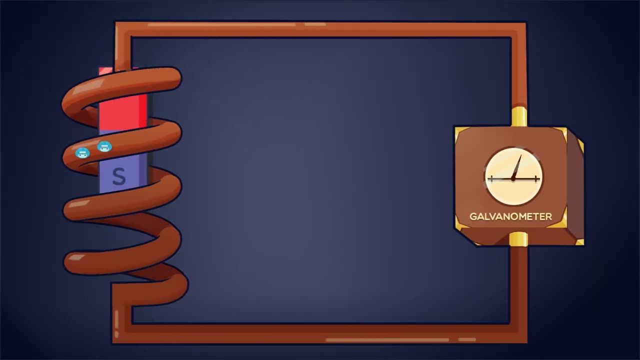 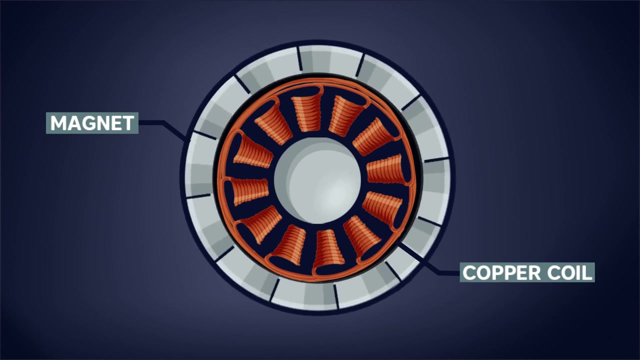 Magnetic induction is the method used to generate most of the electricity worldwide. It all comes down to the way moving magnetic fields affect the electrons in metals. So the next time you plug in, thank all those moving magnets and copper coils and the inventors and engineers who figured out how to combine them to generate electricity. The next time you plug in. thank all those moving magnets and copper coils and the inventors and engineers who figured out how to combine them to generate electricity.